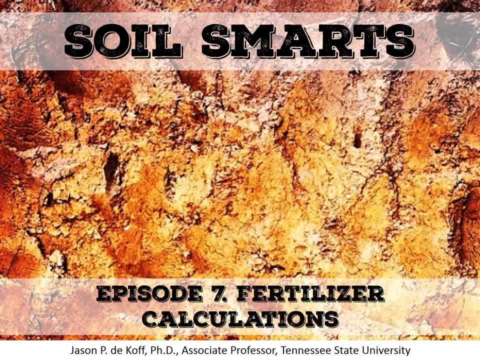 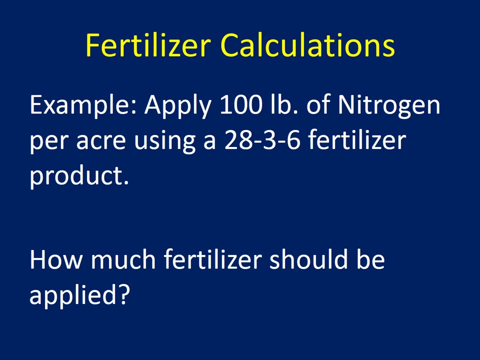 Hi, my name is Jason DeKoff and I'm an associate professor at Tennessee State University. Today, on our Soil Smart series, we're going to be talking about fertilizer calculations. So this is a basic calculation for fertilizer. Somebody wants to apply about 100 pounds of. 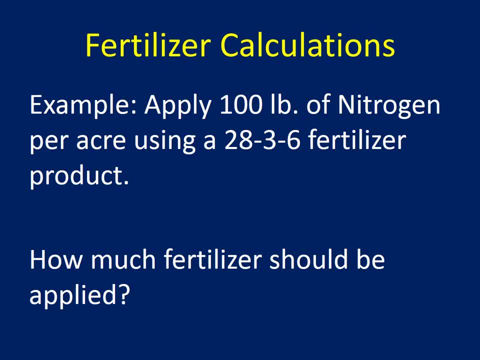 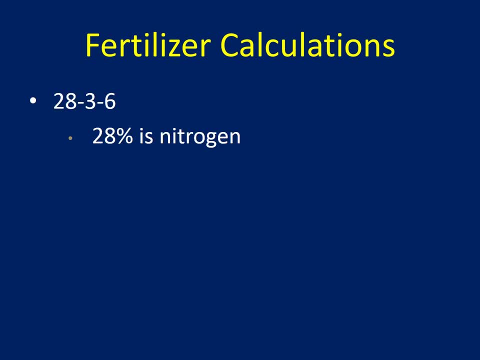 nitrogen per acre and they're using a specific fertilizer product. How much fertilizer should be applied? So the first thing we need to identify is what those numbers mean on the fertilizer bag. The 28 refers to the amount of nitrogen, the 3 represents the relative. 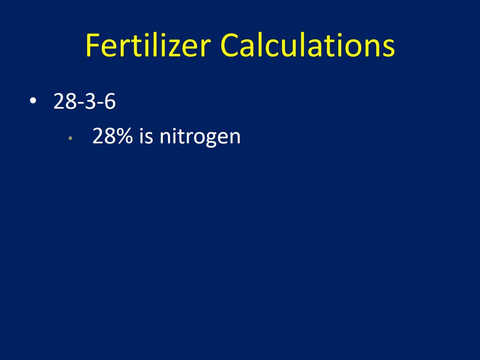 amount of phosphorus, and the 6 represents the relative amount of potassium that's present in that fertilizer. So in this case we're looking at nitrogen. So the 28 means there's 28% nitrogen in that fertilizer. And so the first step we take that 28% and we convert it to a fraction. so we've got. 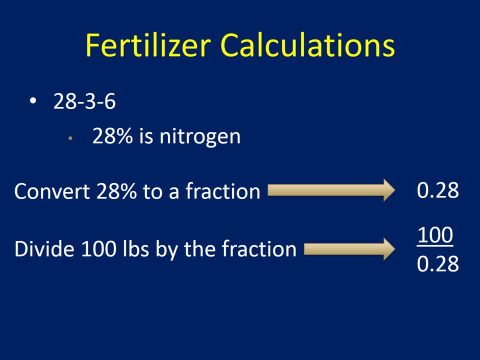 .28.. And then we're going to take that 100 pounds that we need and divide it by the fraction, so 100 divided by .28, and we end up with 357 pounds. So that means we need to apply 357 pounds of that particular product and that will give us our 100 pounds that we are. 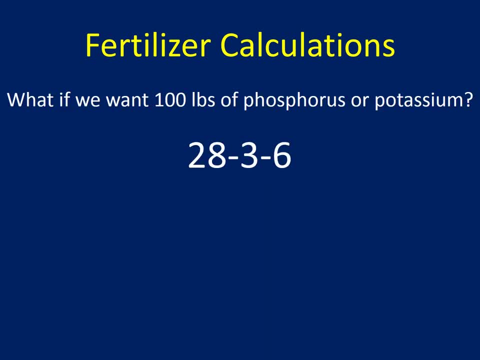 looking for. Now another question: what if we want, say, 100 pounds of phosphorus or potassium? Now, if that were the case, you'd probably want to use a different product than the one we're using, because it has very low amounts of both. But we'll go ahead and use this as an example. 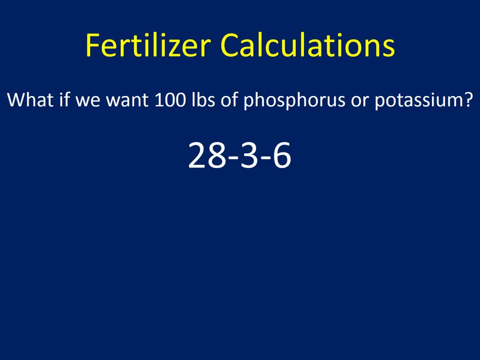 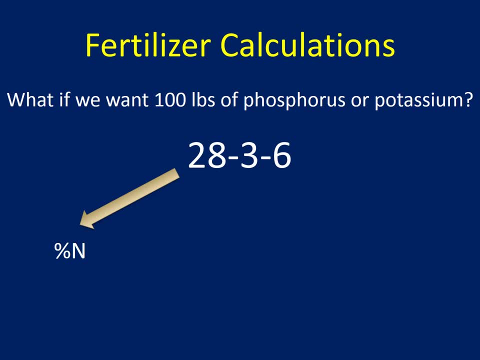 was nice because the 28 that was present in the value represented directly represented 28% nitrogen. Now for phosphorus: the 3% that is shown there actually represents the percentage of P.2O5. So it's not percent phosphorus, it's percent P.2O5.. 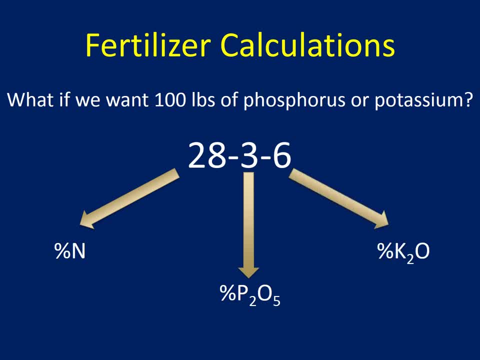 And then also the same thing with potassium. that 6% that we see doesn't represent percent potassium, but it was. it represents percent K2O In there. I was looking at the administration. We'll put this all in the How Actually should. it be? Where is it? Does it value what we do? So we're going to look at Sodiumит first for娘. So we've got 20% here, since we've got 4 individuals. Then obviously you have to take. 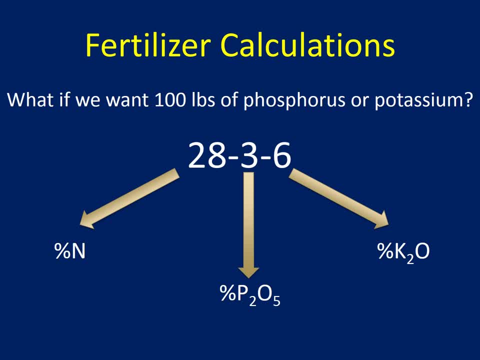 financialistor and you've got to account what's any gain, And so one of the things we have to do, we basically have to go through an extra step of calculation to be able to get to how much phosphorus is actually in the product. 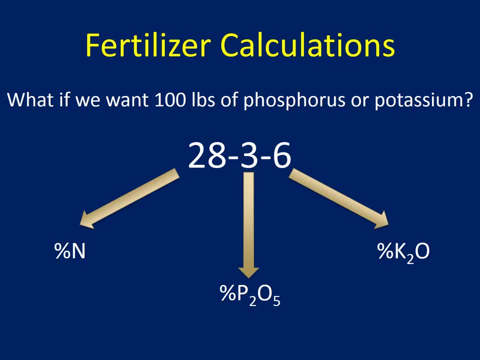 And so to do that, what we do is we identify the amount of phosphorus that's in P2O5.. And for this that's 44%, and that's always going to be 44%. So that's a factor that you can use for any of the phosphorus calculations that you have. 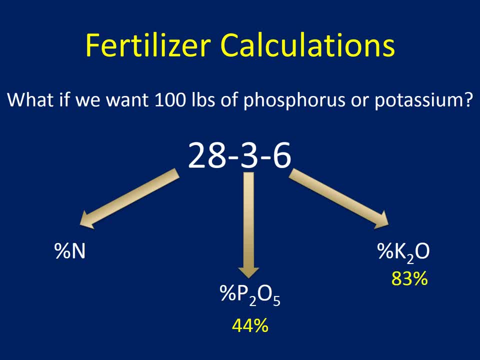 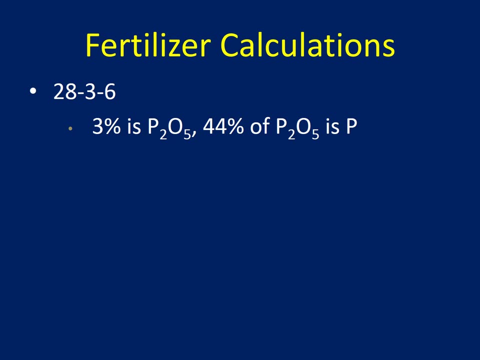 And then for potassium, there's 83% potassium in K2O And so we'll be using these factors- you'll see on the next few slides- for calculating how much we need to apply. So we're looking again at phosphorus And so we know that there's 3% P2O5.. 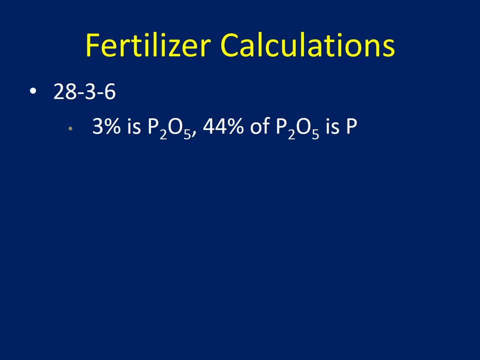 And 44% of that P2O5 is K2O5.. K2O5 is actually phosphorus. So the first thing that we're going to do is we're going to multiply that 3% that's in the fertilizer by 0.44, which is the fraction of that 44% that you see. 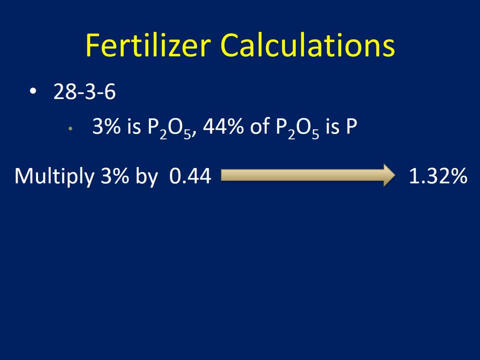 And so we end up with 1.32%. So 1.32% now represents that's how much phosphorus is actually in the fertilizer. So that was that extra step that we had to go through, And now everything else is basically the same as what we did with the nitrogen. 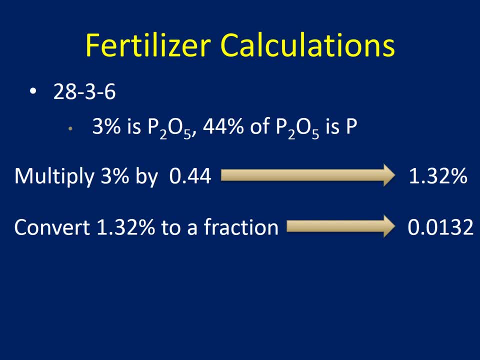 We convert 1.32 to a fraction that you can see there, And then we divide the 100 pounds that we're looking for by that fraction And then we get a value of 7,576 pounds. So, like I said before, you'd most likely be looking for a different fertilizer product. 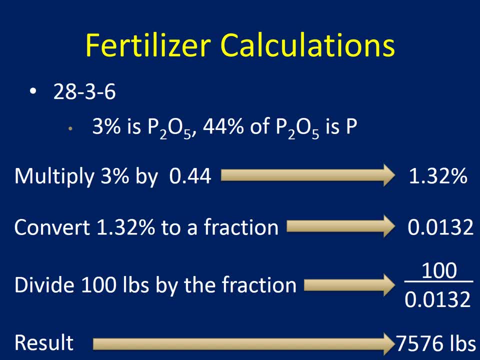 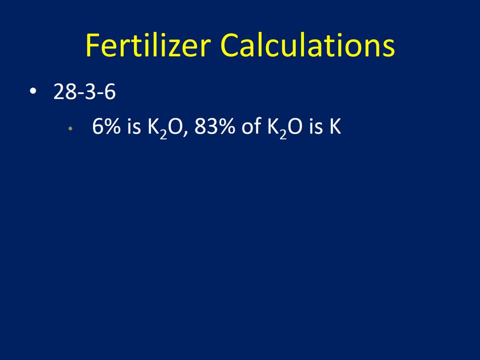 that's got more phosphorus in it to begin with, But this is just for an example, And then. so now this is the one for potassium. Like I said before, 6% of the fertilizer product is K2O. We know that 83% of K2O is potassium.